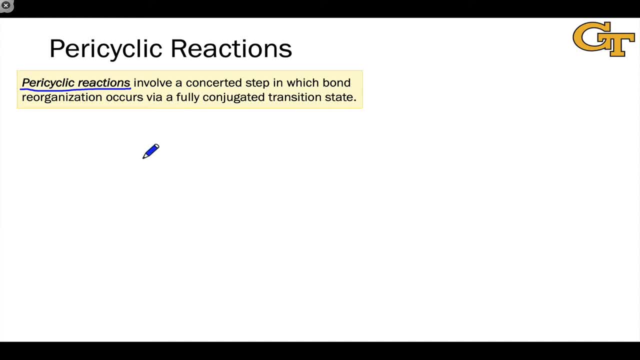 that pericyclic reactions involve a fully concerted step, with multiple bonds forming and breaking at the same time, in which bond reorganization happens through a transition state that is completely or fully conjugated, meaning there's a cyclic array of p orbitals or pi type orbitals spanning all of the atoms involved at the transition state. This idea that the transition state is 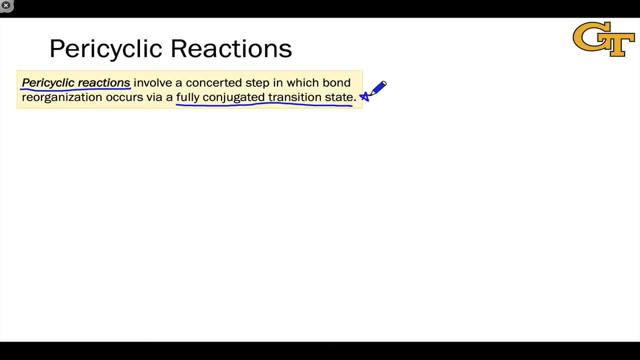 the transition state has to be fully conjugated- actually sets limits on the allowedness of pericyclic reactions and gives us insight into how they actually take place. So it's worth keeping in mind, and we'll apply this idea as we do orbital analyses of photochemical pericyclic reactions. 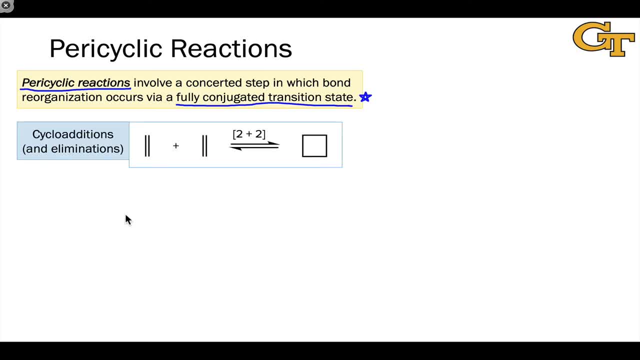 moving forward. There are three types of pericyclic reactions that we'll see. Cycloadditions involve the combination of two separate pi systems to form a ring, and these are named using the size of the pi systems involved. For example, when two two atom pi systems are involved, such as two molecules of 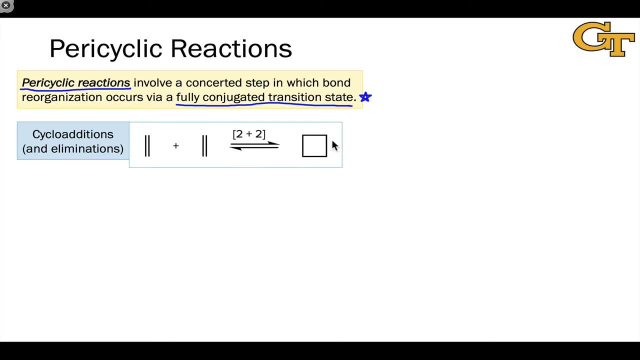 ethylene. like you see here, the cycloaddition is called a 2 plus 2 and the product is a four membered cyclobutane ring. Electrocyclic reactions involve cyclic electron flow within a contiguous pi system of typically an even number of atoms, and these are named using either ring closing. 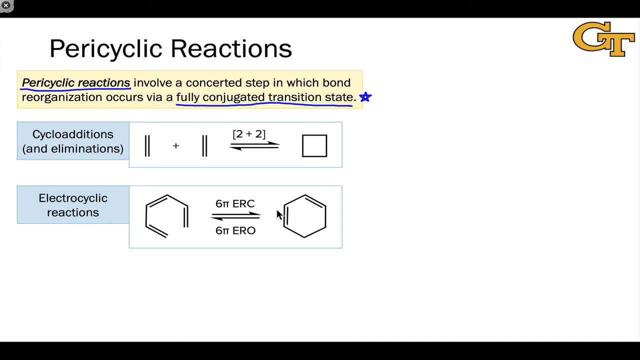 rc or ring opening terminology. so this is a forward ring closing- erc- electrocyclic ring closing, and in reverse it's an ero- electrocyclic ring opening. and six pi here refers to the number of pi electrons involved. six pi electrons, six atoms. it's a six pi erc or six pi. 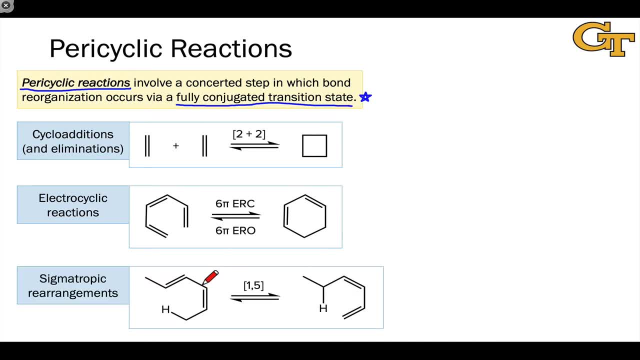 ero process. Sigmatropic rearrangements involve the shifting of a sigma bond from one end of a pi system to another. In a sigmatropic rearrangement, the sigma bond actually participates in the propagation in the transition state and the sigma bonding electrons are actually involved in the 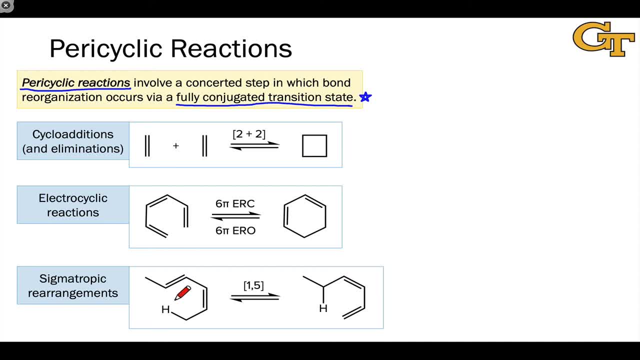 cyclic electron flow. Sigmatropic rearrangements are named using a bit more of a complicated system where we number the atoms on each side of the migrating sigma bond and list those numbers with the smaller first to describe the sigmatropic rearrangement. So for example, here this hydrogen: 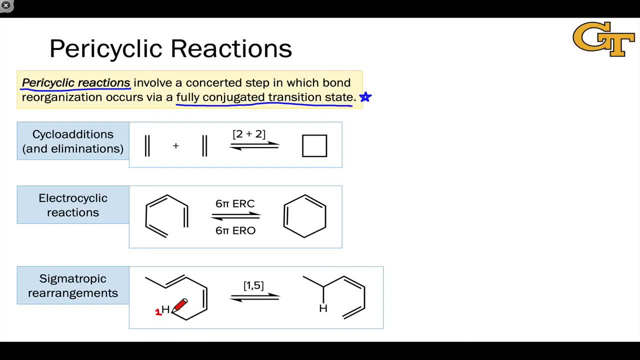 we can label as atom number one on one end of this really key migrating sigma bond, the ch here, and we can number the atoms on the other side, starting with this carbon and working around, including all of the atoms that connect the starting point and the ending point for the. 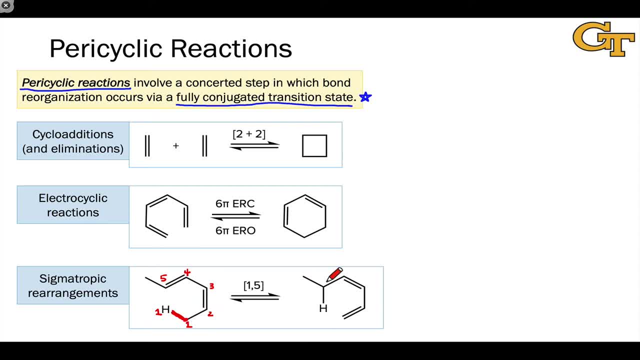 hydrogen. so we go all the way from carbon one to carbon five and we can see that carbon five is where that hydrogen ends up, because the sigma bond migrates from position one to position one on the hydrogen side- there's only one atom on that side- and from position one to position five 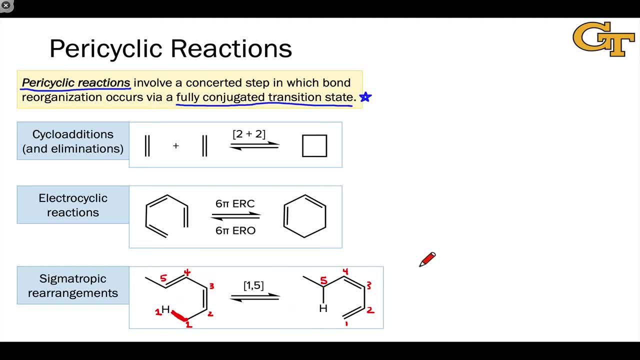 on the carbon side. this is called a one five sigmatropic rearrangement and briefly here, let's draw some curved arrows to depict electron flow in each of these reactions. there are actually multiple ways to do this because of the cyclic nature of electron flow, and that's worth keeping. 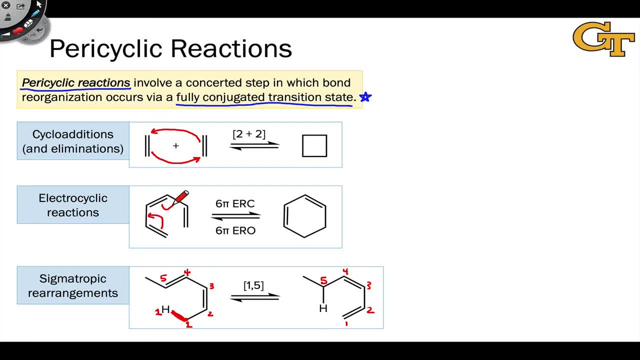 in mind that the curved arrows here are a little bit hand wavy because there are multiple ways to draw them. so we can see in all three cases that we've got electrons moving around in a circle and we can envision a transition state in which all of the atoms are linked and fully conjugated. 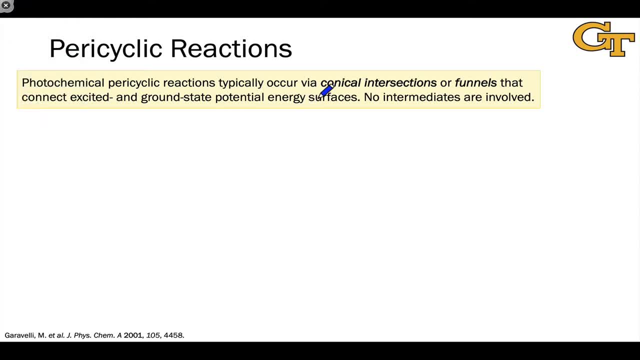 The next point that's particular to photochemical pericyclic reactions is that they commonly occur via conical intersections or funnels. thinking back to our general mechanistic paradigm for photochemical reactions, the way these typically work is there's an excitation to say? 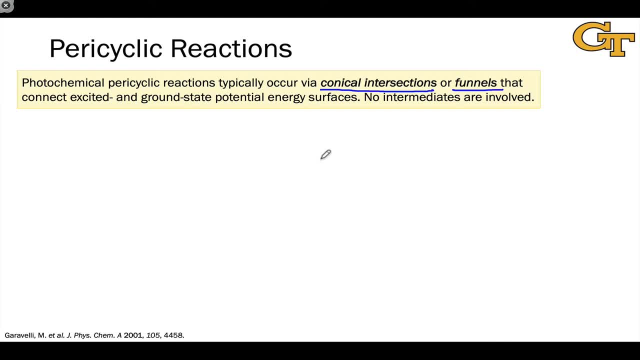 s1. s1 returns to the ground state, potential energy surface through a very rapid movement through a conical intersection or funnel. most commonly in photochemical pericyclic reactions no intermediates are involved- reversal. but it's a good starting point. it's a good zero-order guess. 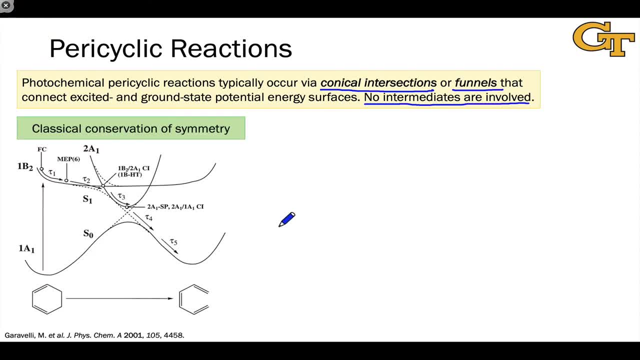 So to remind us what a conical intersection looks like on a potential energy surface diagram, I actually want to start with this diagram from this paper by Garavelli, where he draws a sort of classical potential energy surface diagram for the photochemical ERO process. 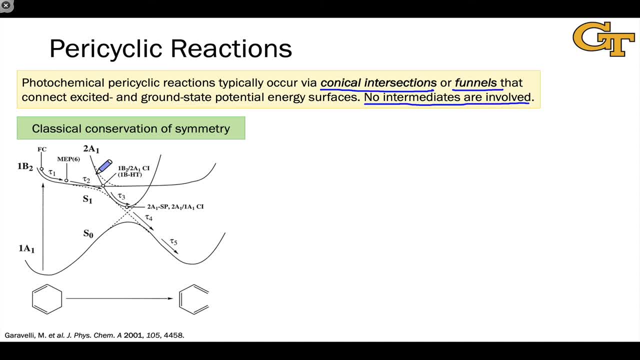 of cyclohexadiene. We can identify a conical intersection here where the 2A1 potential energy surface crosses the 1B2 potential energy surface, and we can identify here a funnel with a qualitatively different structure where there is what we call an avoided crossing.